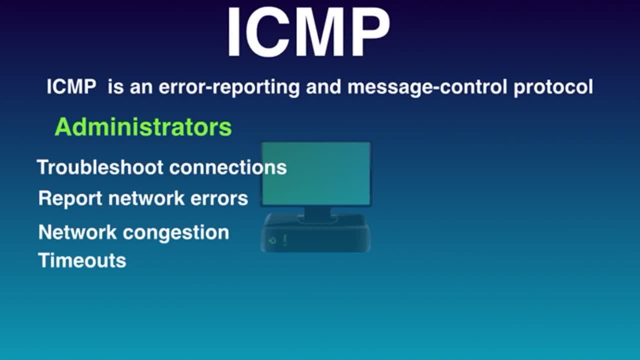 Basically, ICMP is used to diagnose network issues and determine whether or not data is reaching its intended destination in a timely manner. In order to maintain the security and safety of networks, maintaining a successful communication between devices, ICMP is necessary. Let's put it this way: ICMP is a transport level protocol within TCP IP network that transmits 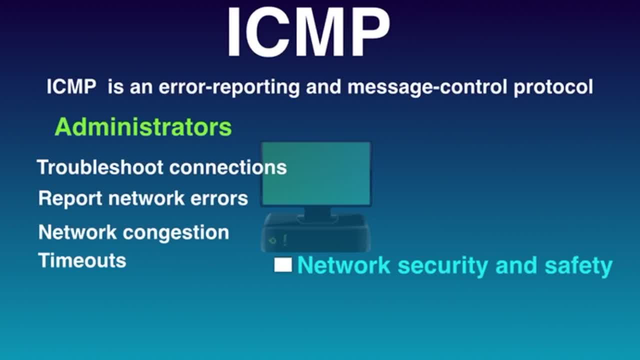 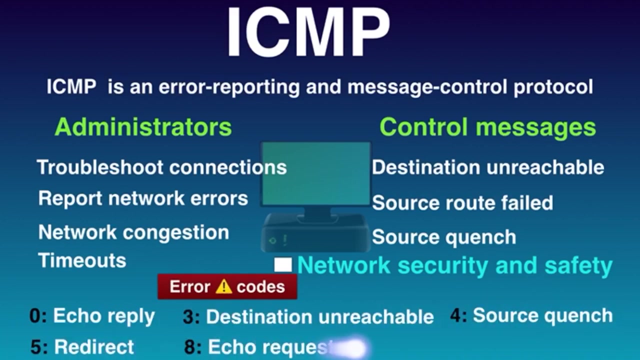 information about network connectivity issues back to the source of the compromised transmission. It sends control messages such as destination network unreachable, source root failed and source quench. These are some ICMP error codes. Echo reply: destination is unreachable, source quench. 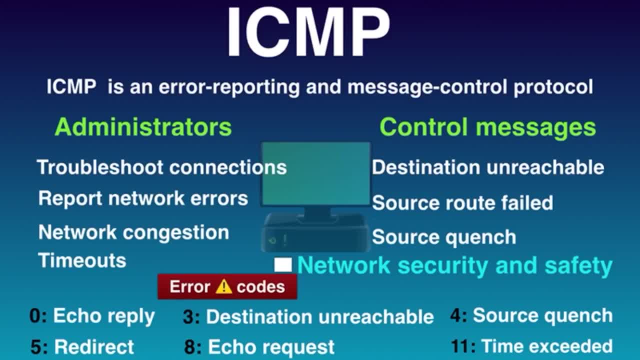 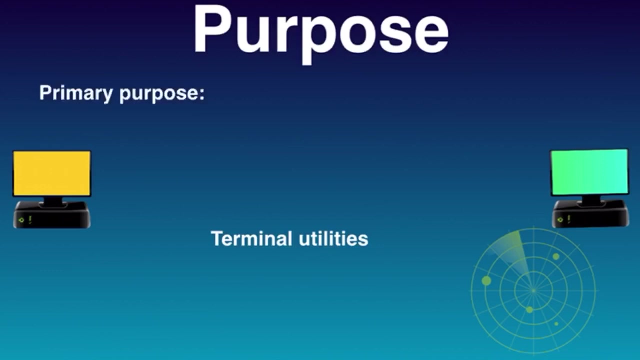 redirect echo request. time exceeded. Echo request are similar. Used for ping. Time exceeded. It is used for trace route. Source quench means router is overloaded. Let's talk about the purpose of ICMP. Primary purpose of ICMP is for error. 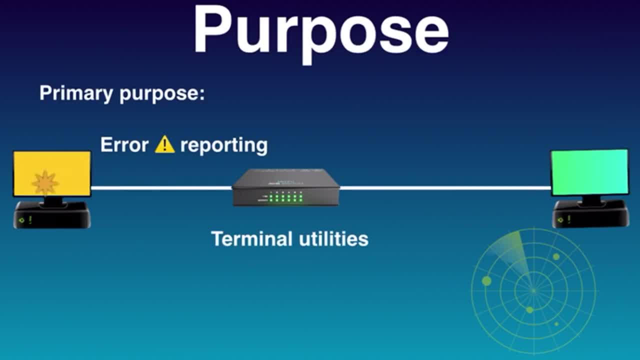 reporting. When two devices connect over the internet, ICMP generates errors to share with the sending device that any of data did not get to its intended destination. ICMP is used for error reporting. Primary purpose of ICMP is for error reporting. When two devices connect over the internet, ICMP generates errors to share with the. 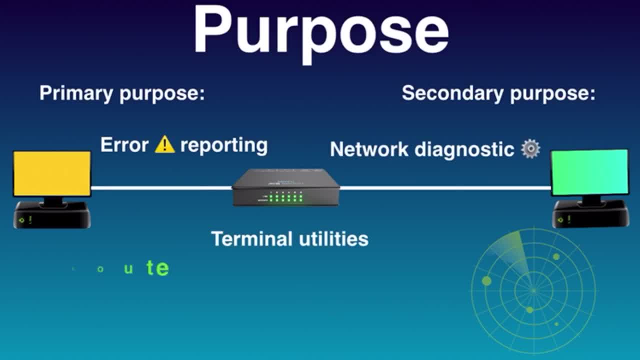 sending device that any of data did not get to its intended destination. Secondary purpose of ICMP protocol is to perform network diagnostics. Commonly used terminal utilities- trace route and ping- both work using ICMP. First we will get to the details of ICMP. First we will go to the first part of the. 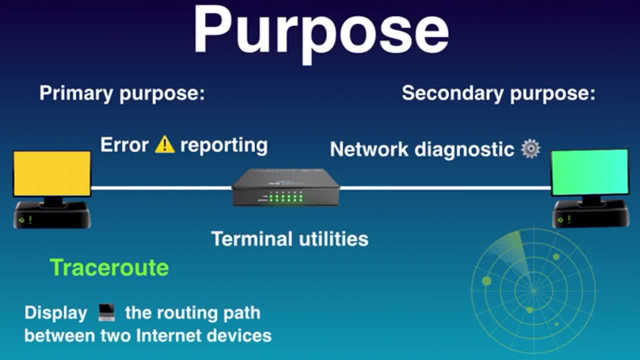 that a request must pass through before it reaches its destination. ping utility is a simplified version of traceroute. a ping will test the speed of the connection between two devices and report exactly how long it takes a packet of data to reach its destination and come back to the center's device. when we do a ping command, it creates an echo request and expect.